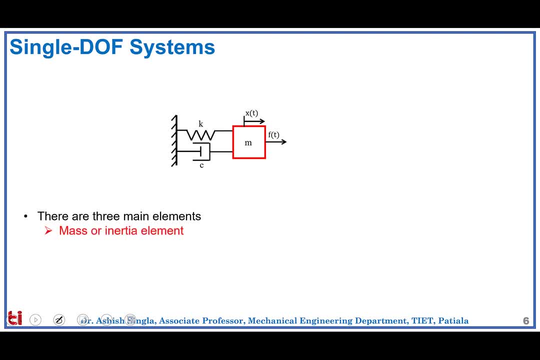 Mass or inertia element, which is basically tries to oppose the translatory motion of the body. The second element is the spring element, which is basically energy storing element and it stores the strain energy because of its deflection. The second element is the spring element, which is basically energy storing element. 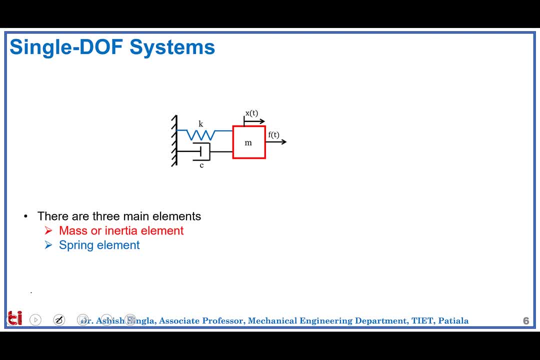 which stores energy as strain energy because of its deformation, And the natural tendency of the spring is to retain its original position And that's why it tries to oppose the displacement. Whereas the third element is the damper element, which basically represents the amount of energy being dissipated by the system. 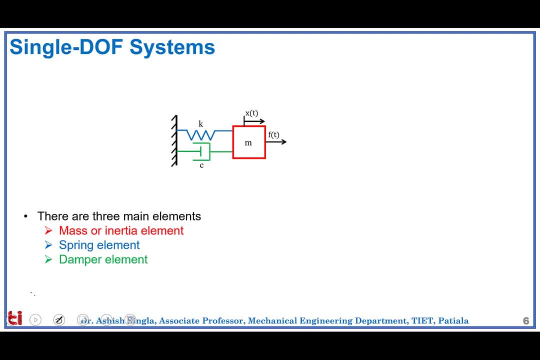 This may be because of friction, this may be because of air drag, this may be because of a resistance, And it is called as the viscous damping, where the tendency of the damper is to oppose the velocity of the body. So, in order to develop this equation of motion, of this single degree of freedom system, we need to follow some steps. 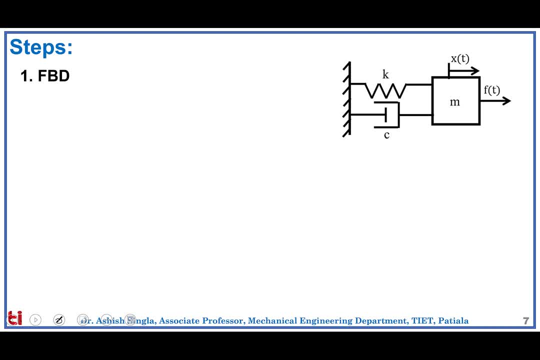 The first step is called as the free body diagram, where we need to isolate the body and we need to show all the forces being applied on the system. So let's say the body is under the influence of external force, Ft, So as the force is being applied to the right side, so shown like F of t. 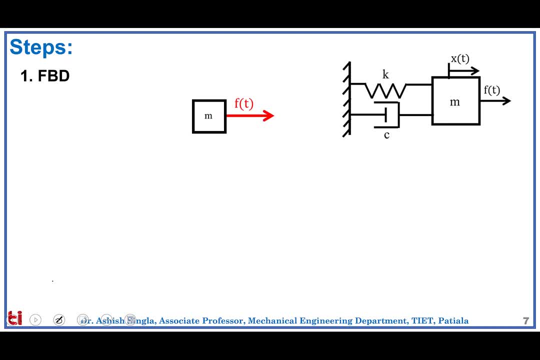 So, under the influence of this force, the spring K is being stretched and, as mentioned earlier, the tendency of the spring is to regain its original position. So the spring will apply a backward force towards the left hand side, which is called as Kx. 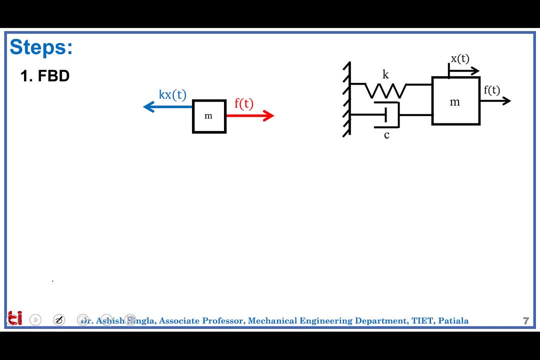 This is the force being applied by the spring. Similarly, the tendency of the spring is to oppose the velocity, So the damper will apply a force Cx towards the left hand side in order to oppose the velocity of the body. 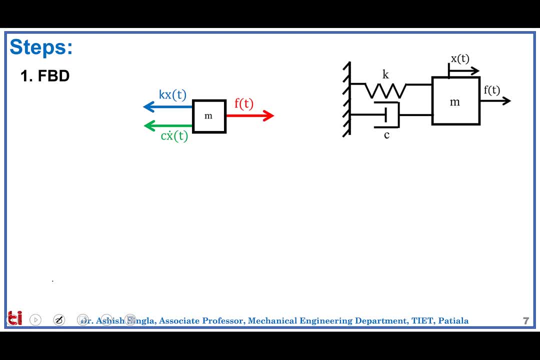 So this is the free body diagram, where all the forces acting on the body have been marked. Now we need to apply the Newton's second law of motion, which shows that the rate of change of linear momentum of the body is equal to summation of all the forces acting on the body. 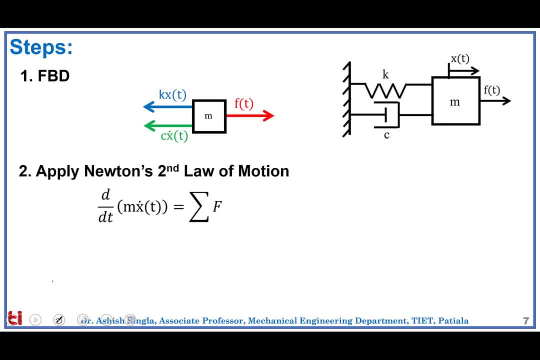 So under d by dt, we can apply the UB formula of differentiation, which shows that m dot, x dot plus mx double dot should be equal to summation of all the forces acting on the system. So in 95% of the cases the mass of the system will remain constant. 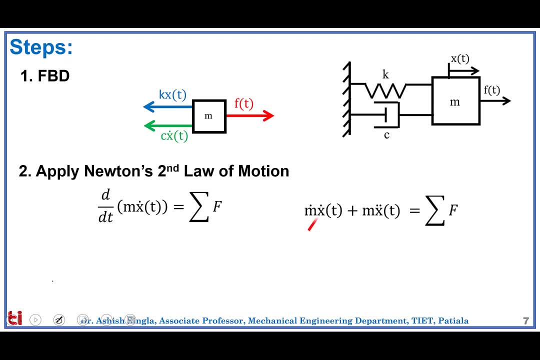 So this term will go to zero, Whereas in some cases, like you can say, take the example of a missile which is going to hit the aircraft. So in that case, this assumption is true. This assumption is not valid because the rate of change of mass 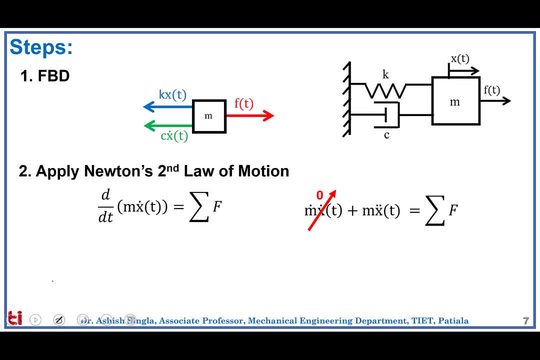 in the case of a missile is significant and we cannot assume this kind of assumption. But otherwise, in all normal systems, we assume that the mass variation is negligible, So that's why rate of change of mass can be assumed to be zero. 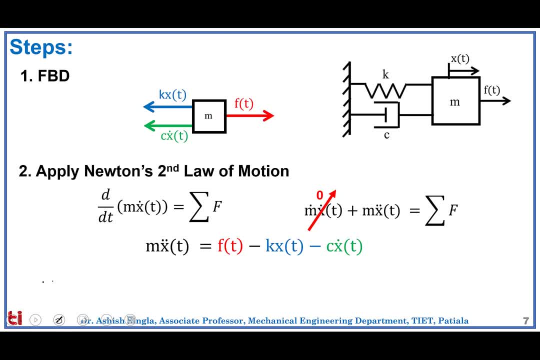 So, which means mx double dot, should be equal to summation of all the forces acting on the system. So we will assume all the forces acting on the right hand side to be positive and all the forces acting on the left hand side direction are negative. 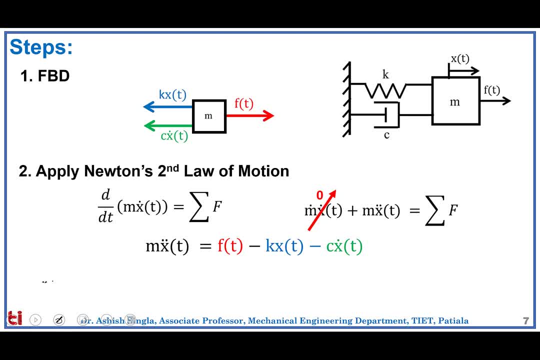 So that's why ft minus kx minus cx dot, So, on collecting the terms, we have mx double dot plus cx, dot plus kx is equal to f of t, which is the standard equation of motion of the spring mass tamper system. 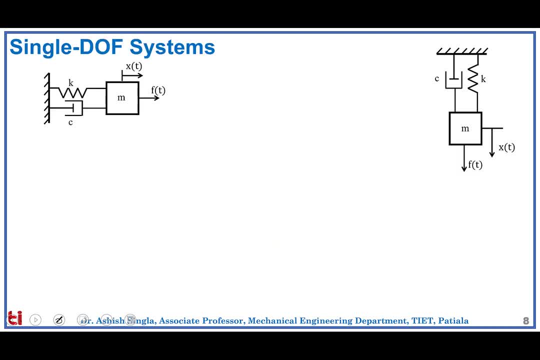 Now let's try to orient the body. So earlier we have considered the body in the horizontal direction. Now let's try to orient the body and let the body is in the vertical direction. Let's see if there is any change in the equation of motion. 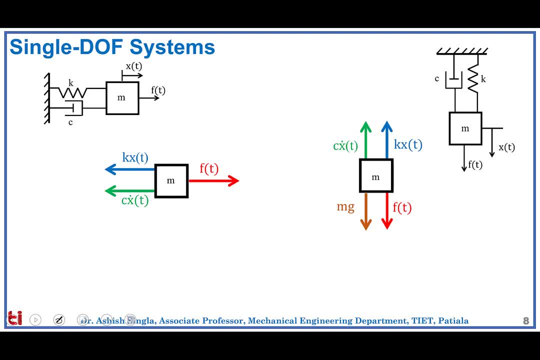 because of this change in orientation. So this is a free body diagram. So this is a new free body diagram of the body in the vertical direction, where we can say: now the mg force will also come into play. So because of this mg force, there is a change in the equation of motion. 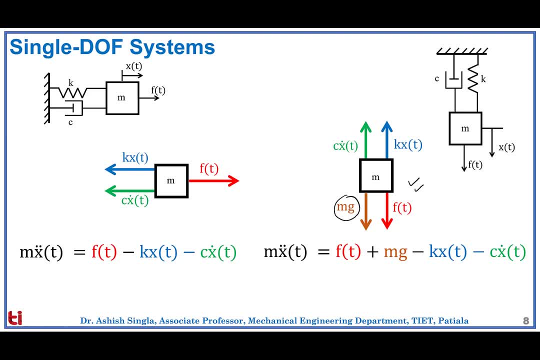 So now this mg factor will come into play, So which will be shown over here. So because of this mg, you can see there is a change in the equation of motion of the original system. So because of this mg, you can see there is a change. 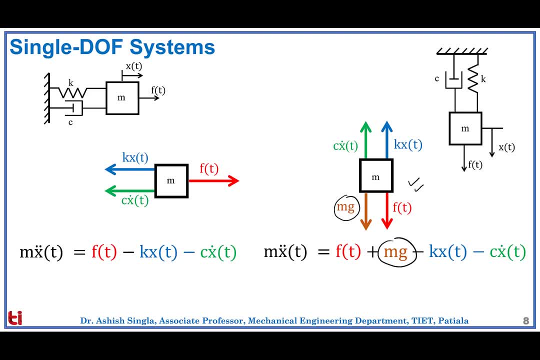 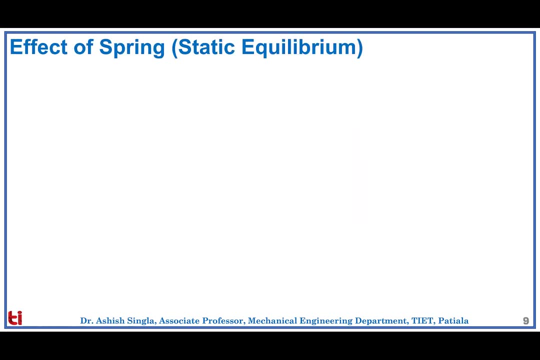 in the equation of motion of the system. so is it the correct equation or no? so let's figure out. on collecting the terms, we will find the equation to be like this way, but this is not the correct equation. so let's try to find out the reason why. so we need to understand the effect of spring, or you can say the. 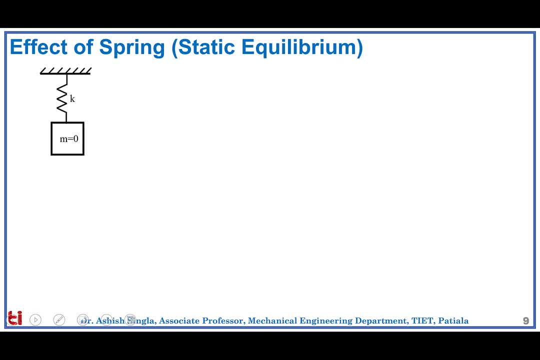 effect of static equilibrium. so let's say, when the spring is suspended with no mass on this, so the spring is having some free length, as we suspend a mass M, the spring will vibrate and comes to the static equilibrium configuration after a elongation of Delta static. so you can see, after we apply a mass M now the 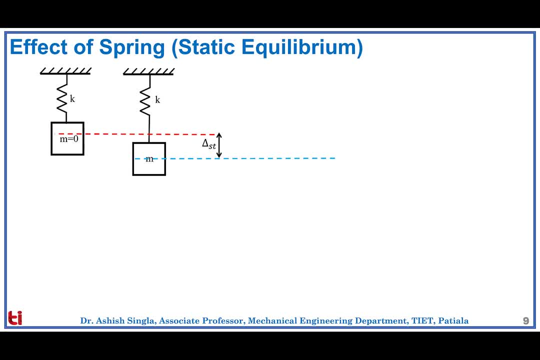 spring has already elongated by amount Delta static. so at this position we can draw the free body diagram and we can see that the mg force has been compensated by the elongation of the spring. so we can see this: mg is equal to K Delta static. so now, under the influence of this force, 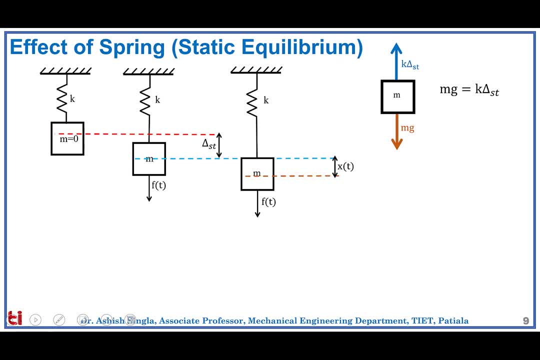 F' ≥ y' ≥ ≥ k'. Now, under the influence of this force F' ≥ y'≥ k'. now, under the influence of this force F', the spring will further elongate by xt, So the total elongation of the spring. 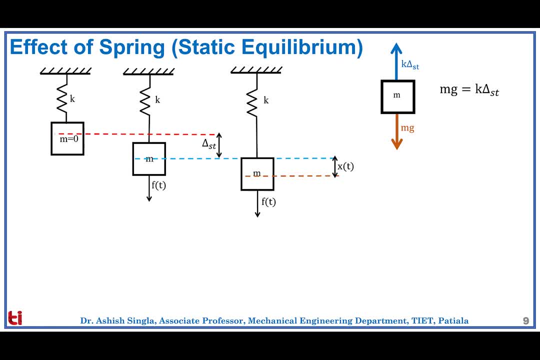 you can see from the original mean position is xt plus delta, static Now if we draw the new free body diagram. so here you can see we have mg force, we have this ft external force and we are having this spring force where the 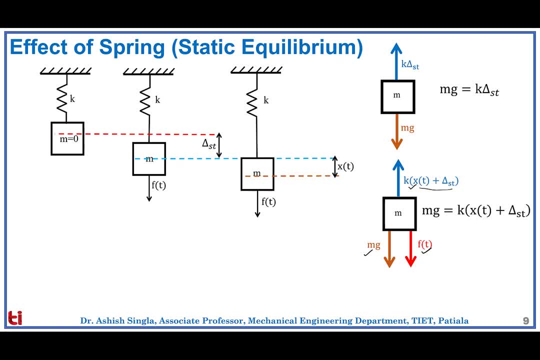 spring has been elongated by xt plus delta static. So if we now write the terms- so here you can see- the mg force will be cancelled with k-delta static from the equilibrium condition. So after cancelling both the terms, you can see. 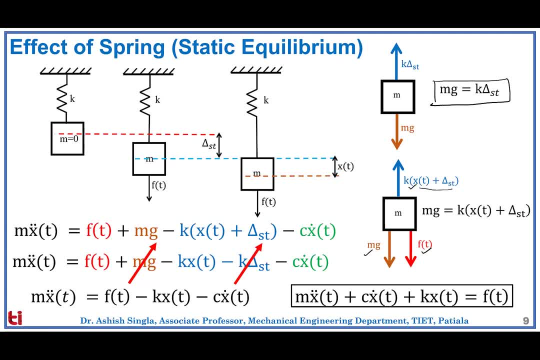 the original equation is intact and there is no change in the equation of motion of the original system. So the reason being that we have defined in the previous slide that xt, the displacement, is not a normal displacement. it is the displacement from the static equilibrium configuration, which means after the 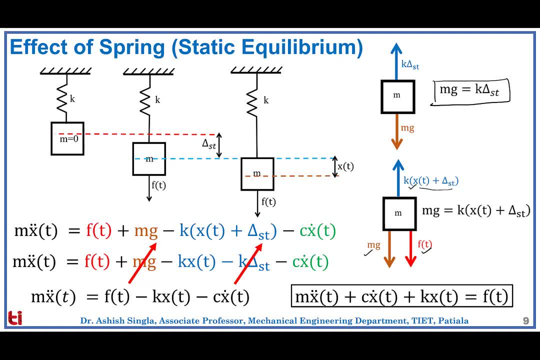 spring has elongated where it has already balanced the mg force. So there is no point in considering these two forces along and then keep on cancelling every time. So by simply saying that the xt is the displacement from the static equilibrium configuration, we can simply neglect the mg term. So then comes the 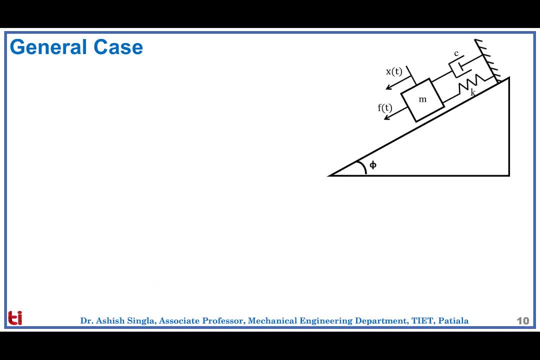 general case. So here you can see, there is a body which is on inclined wedge. So again, we are having a spring, having stiffness k, there is a damper of damping coefficient c and the body is under the influence of the force ft due. 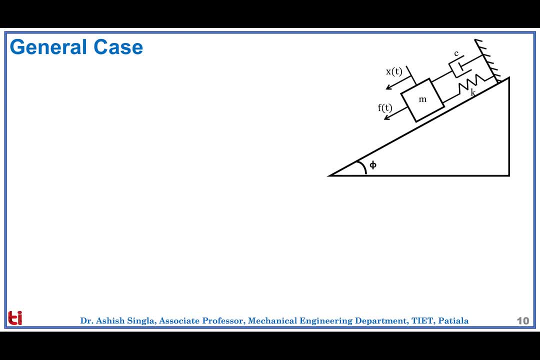 to which it is having displacement xt from the static equilibrium configuration. So now over there we can again apply the condition. So here you can see, this is a force mg, this is mg cos phi and this is mg sine phi. So under: 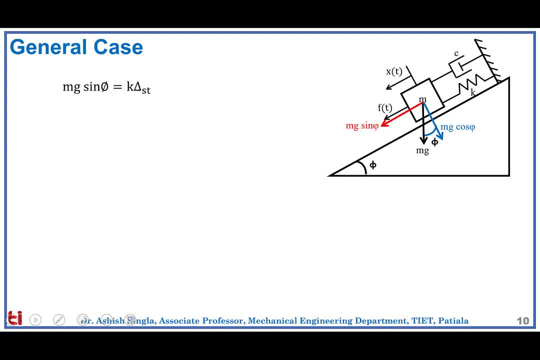 static equilibrium. this mg sine phi will be counterbalanced by the k-delta static. So this is a new equilibrium condition in this particular case. So again, if you look at the same set of equation, we will see that this mg sine phi will be. 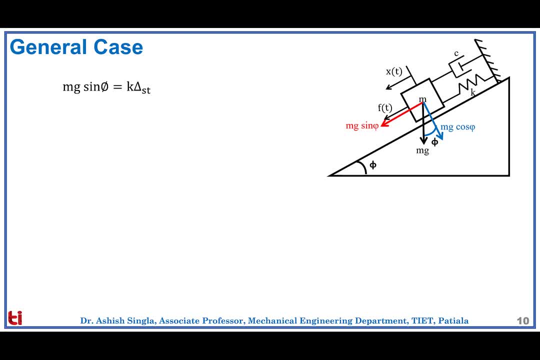 cancelled with k-delta static in the final equation and eventually you will get the same equation back. So you can see this. phi represents basically the set of all cases When phi is equal to zero. we have the horizontal case When phi is equal to 90, we are having the vertical case which we have discussed in. 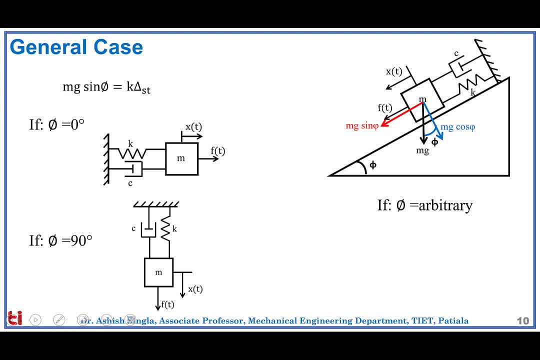 the last slide and when phi is arbitrary, we have the inclined case. So in all three cases we can see the equation of motion will remain the same. So what is the crux? We can see whenever there is a spring, either vertical or inclined, we need not to consider the mg force. 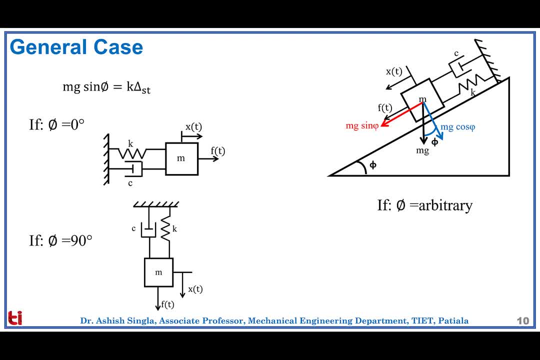 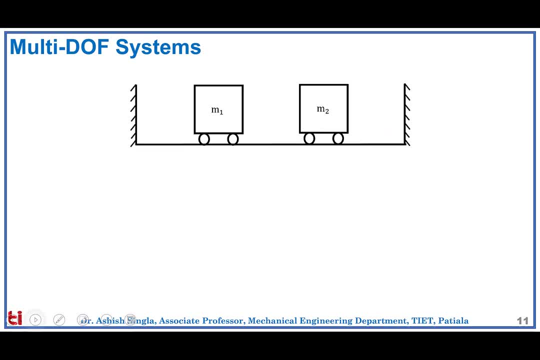 because that has already been compensated by the spring element. So now comes the multi degree of freedom systems. So let's consider a two degree of freedom system having two masses, m1 and m2.. Let's say these two masses are connected by three interconnected springs having stiffness: k1, k2, k3 and 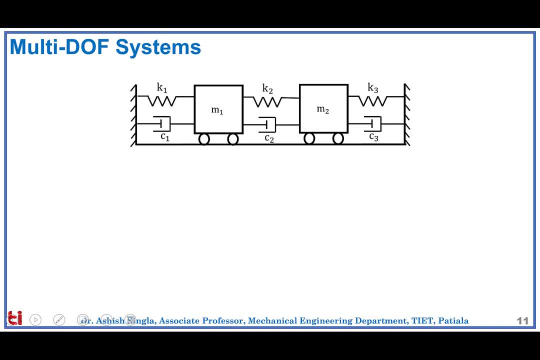 they are also attached by three dampers having damping coefficients as c1, c2, c3. So both the bodies are under the influence of external forces, f1 and f2 respectively, and they are being displaced by x1 and x2 from their 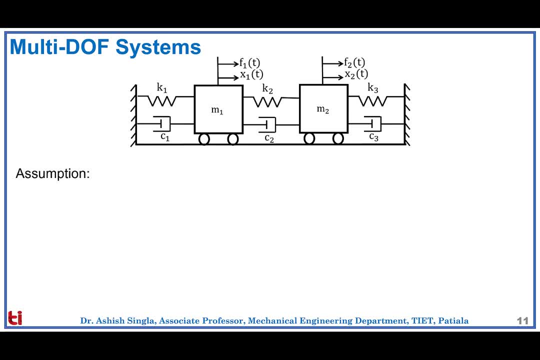 respective static equilibrium positions. So, in order to develop the free body diagram of such kind of systems, we have to assume whether x1 is more than x2 or x1 is less than x2 in order to draw their free body diagrams. So the three 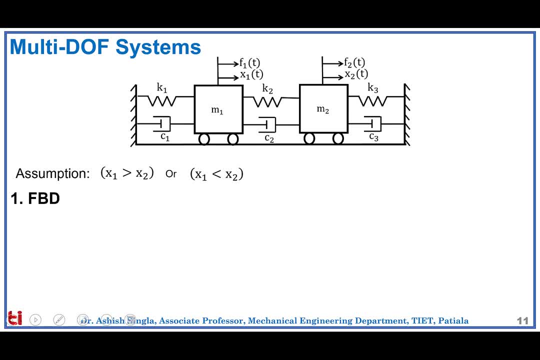 force fotografies are given in this diagram and x1 is less than x2.. The two forces are beginning to change In order to determine the free body diagrams we need to do correctly, so let's try to see this. so, first of all, we need to develop the free 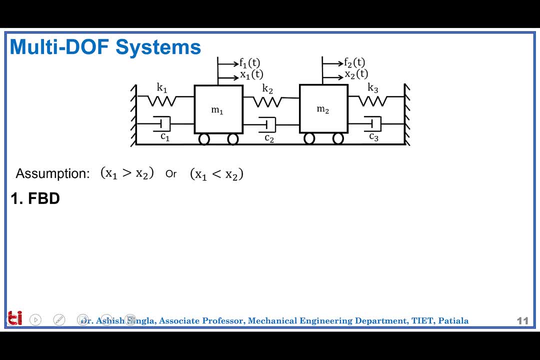 body diagram. so in multi degree of freedom systems, it's always advisable to draw the free body diagram of both the bodies simultaneously. so let's draw both the bodies, M1 and M2. so first of all, let's consider this spring K1, which you can see. one end of the spring is fixed, whereas the other end of the spring is. 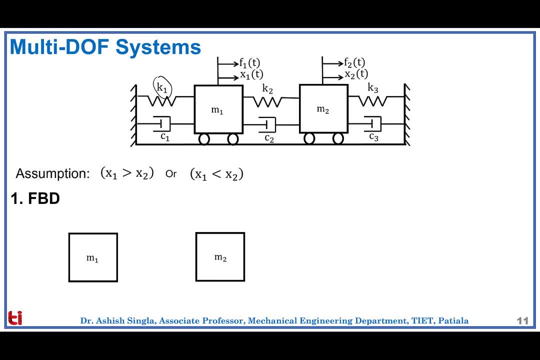 attached to the moving body M1. so under the influence of force F1 which is up being applied on the first body on to the towards the right hand side. you can see, as the body goes to the right, the spring K1 is stressed and it will. 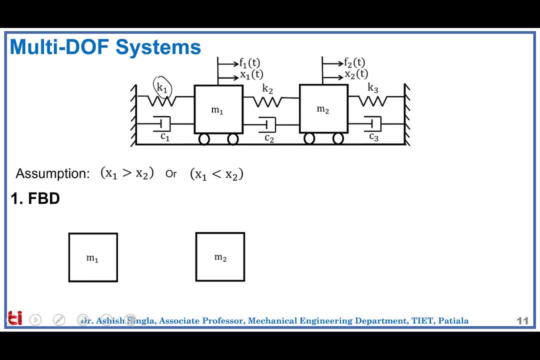 apply a backward force onto the body which is equal to K1 x1.. The similar is the case with spring K3, because the body M2 is under the influence of force F2 towards the right hand side. so as the body M2 moves to the right, the spring 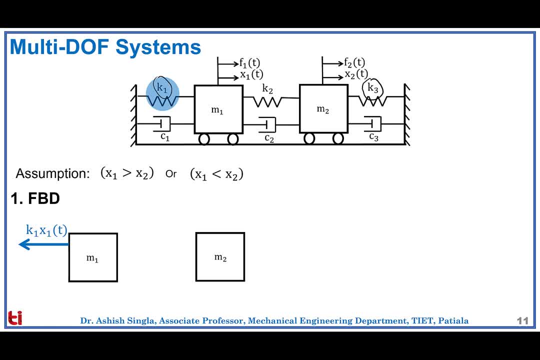 K3 is being compressed and the tendency of the spring is to regain its normal position, So that's why it will try to oppose the motion x2.. Thus it will apply outward force on the m2 body, that is, towards the left, which is equal. 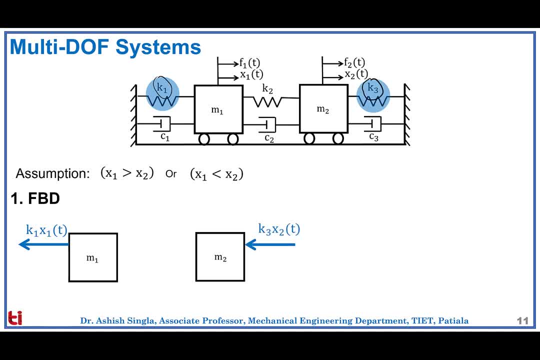 to k3 x2.. Similar things will be applied by a damper c1 and c3. So the force applied by the damper on the first body is c1- x1 dot, whereas the force being applied by the damper c3 on body m2 is c3- x2 dot. So these two cases are pretty. 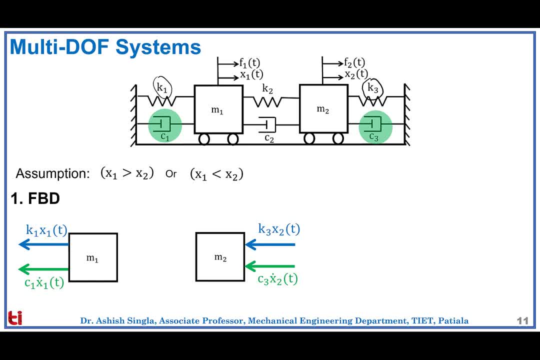 simple because in both the cases you can see, one end of the spring is fixed, whereas the other end of the spring is connected to a moving body. Now comes to the spring k2, which is called as a coupled spring. In this case, you can: 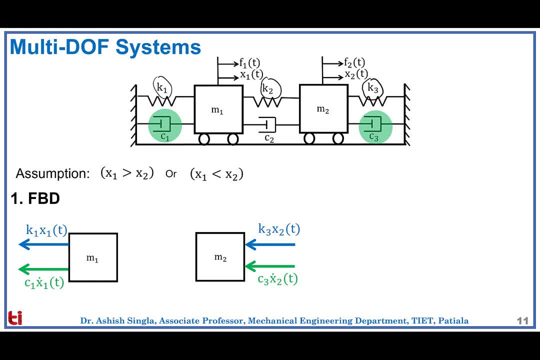 see, both the ends of the spring are attached to movable bodies. That's why it is called as a coupled spring. So under this condition, in order to develop the forces correctly, we have to assume whether x1 is greater than x2 or x1 is. 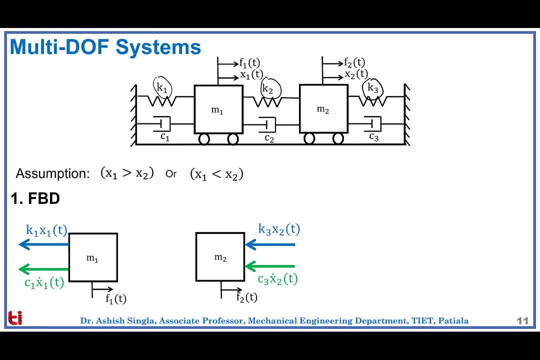 less than x2.. So let's take the first case, where x2, X1 is greater than X2 under the influence of two forces, F1 and F2.. So here you can see as both the bodies move to the right, as shown in this figure, as both 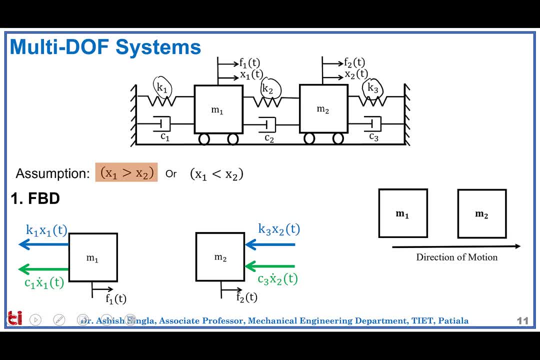 the bodies move to the right and with X1 is more than X2, the bodies will eventually come closer to each other, which means that the K2 spring is compressed and it will apply outward force on both the bodies and the magnitude of force is K2 into X1 minus X2, because X1 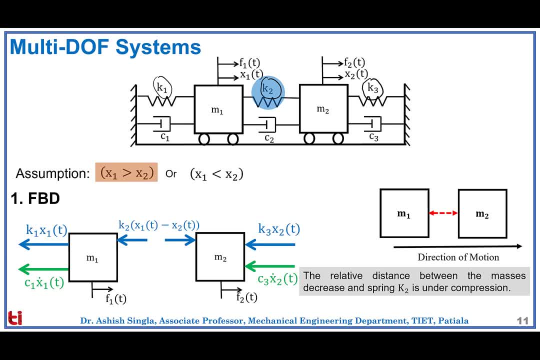 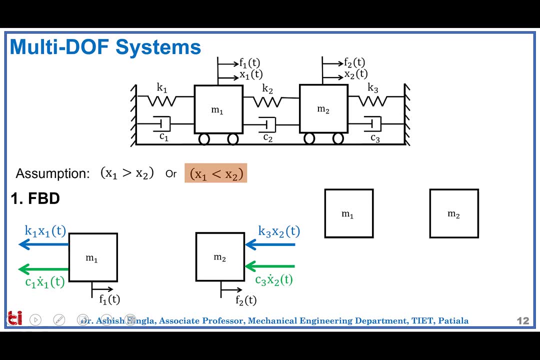 is greater. so that's why we have K2 into X1 minus X2.. The similar is the tendency of the damper. so we have the force due to damper is C2 into X1 dot minus X2 dot. Let's consider the next case, when X1 is less than X2, so under this case, so as X1 is less. 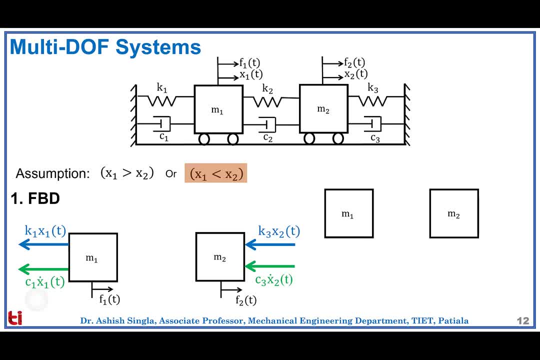 than X2 and both the bodies are moving towards the right. We can see that The distance between the bodies will increase And the state of the spring K2 is stretched. so as K2 is under tension, it will apply inward force on both the bodies. it will pull both the bodies towards itself. 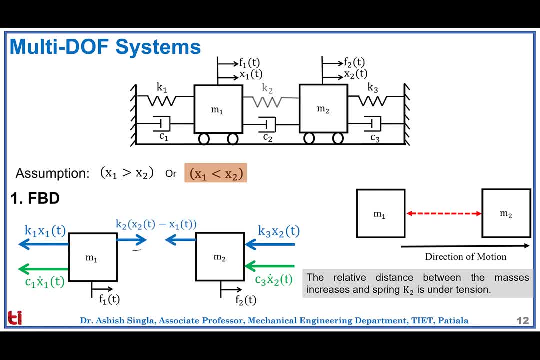 And that's why the direction of these two arrows have changed. now, And also you can see the force applied by the spring is K2 into X2 minus X1, because now X2 is more than X1.. The similar thing is applicable for the damper. 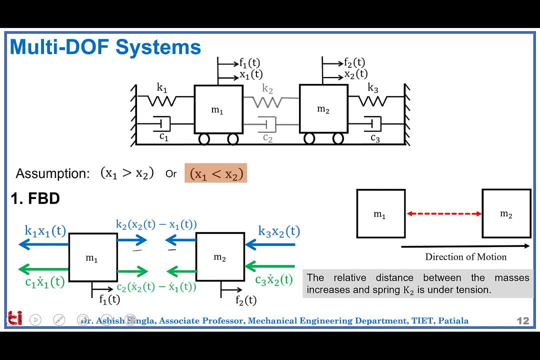 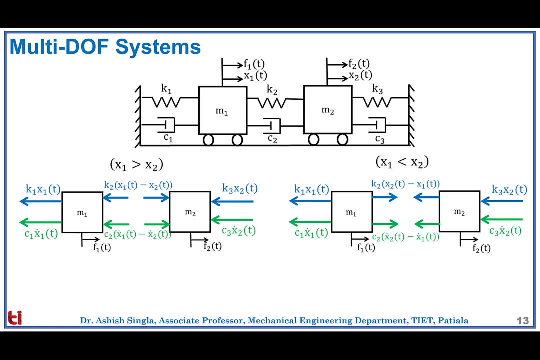 And the damping force can be written as C2 into X2 dot minus X1 dot. So here both the free body diagrams are placed side by side. The first case is the. on the left hand side we have X1 greater than X2.. 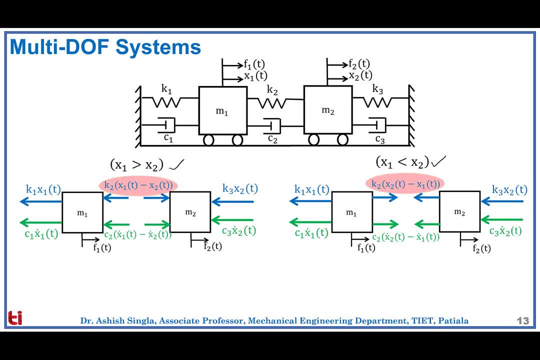 On the right hand side we are having X1 less than X2.. So under both the assumptions you can see there is a change in the sign over here. Here it is X1 minus X2, here it is X2 minus X1, and also there is a change in the direction. 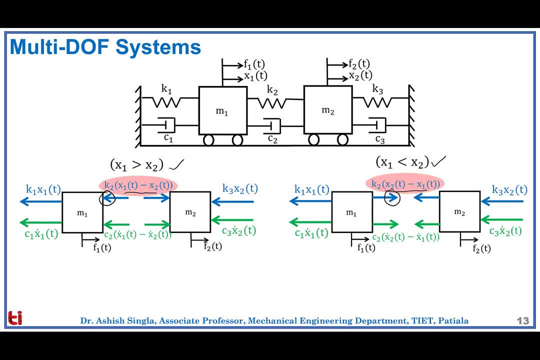 of the arrow. So these minus sign in the direction of arrow, So these minus sign in the direction of arrow, So these minus sign in the direction of arrow, will counterbalance each other. So eventually you can see that the equation of motion will turn out to be same. 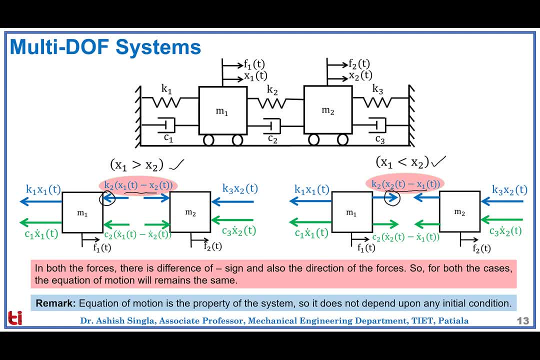 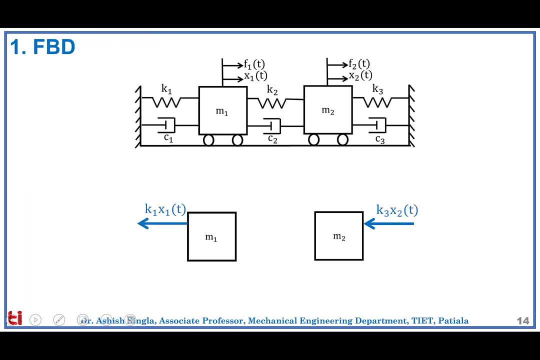 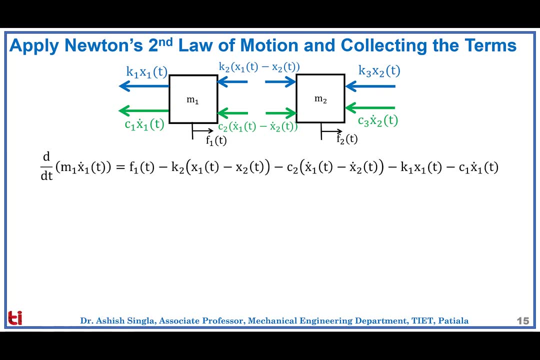 So, which means that equation of motion is a property of the system and it does not depend upon any assumption, as well as any initial condition. So now let's try to develop the free body diagram. So on collecting the terms we can see. so, after developing the free body diagram, next, 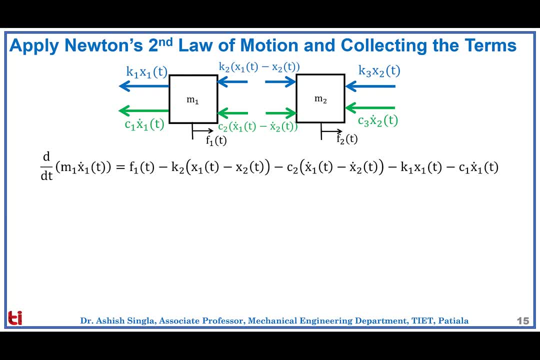 we need to apply the Newton's second law for the first body, which shows that rate of change of linear momentum of the first body, that is, M1, X1 dot, should be equal to summation of all the forces acting on the first body, which is equal to F1 t minus K2, into X1 minus. 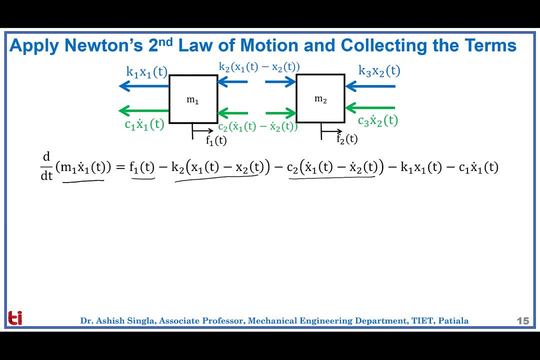 X2 minus C2 into X1 dot minus X2 dot minus K1, X1 minus C1, X1 dot. So, after collecting the terms, similarly we can write the equation of motion of the second body where the rate of change of linear momentum of the second body, that is, M2, X2. 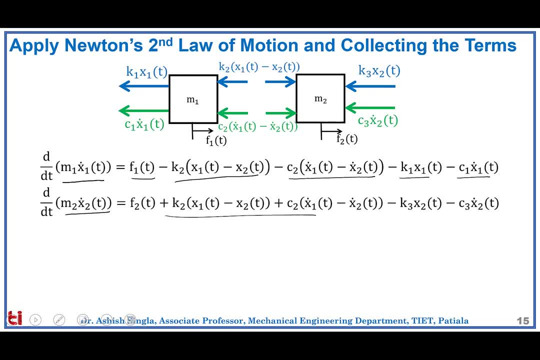 dot. So we can do this expression. So now we can collect the terms For the first equation. we have M1, X1 dot plus C1 plus C2 times X1 dot minus C2, X2 dot plus K1 plus K2 times X1 minus K2, X2, equal to F1 of t. 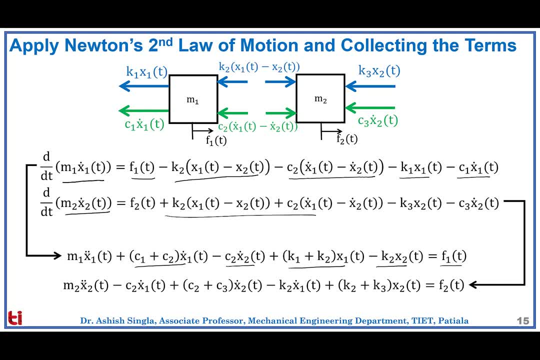 And for the second body we have M2 X2 double dot minus C2 X1 dot plus C2 plus C3 times X2 dot minus K2 X1, this dot should not be there- plus K2 plus K3 times X2.. 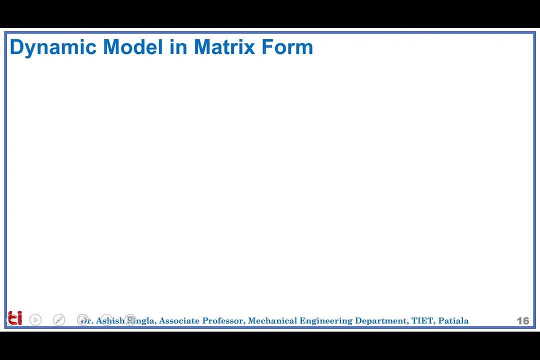 So this is the expression. So, after developing equation of motion of both the bodies, we are now in a position to write them in matrix form. So let us see the structure of the equation. So this is the representation of the dynamic model in matrix form which you can see having. 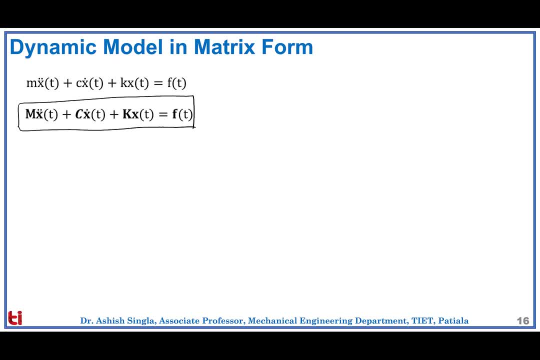 one to one correspondence with the equation of motion written in the scalar form. So here you can see, M is a scalar, whereas this M is a matrix. Similarly, you have C and K are scalars over there, Whereas this C and K are scalar. 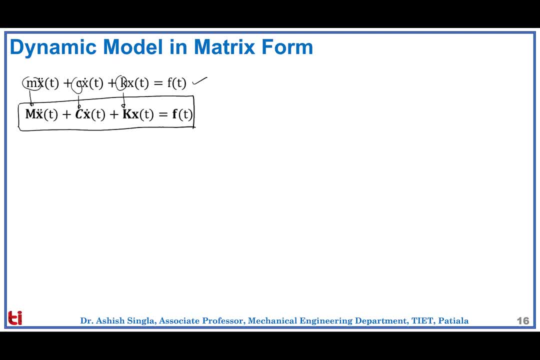 So this M is a matrix. Similarly, you have C and K are scalars over there And K are matrices over there, And this X of t is the displacement of the single body, whereas this X of t represents the vector of displacements. 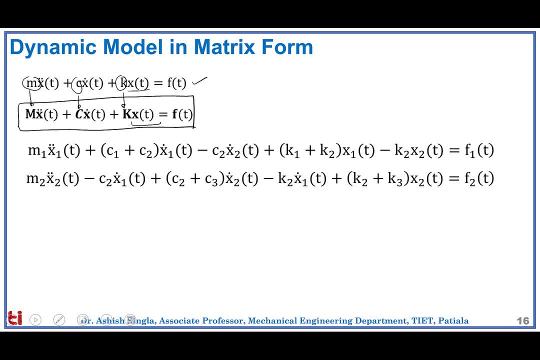 So let us rewrite both the equations. Now we have this. so for this two degree of freedom system, we have this Xt vector as having components X1 of t and X2 of t, which is written over here as vector of displacements. 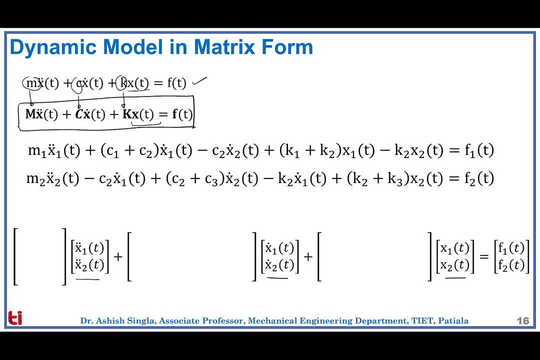 vector of velocities, vector of accelerations, And here we have the vector of displacement. So let us write both the equations. So we have T denoted as T shortcut, and T, So in order to write 2 and 1 vector of forces. so now we can write the matrix form. 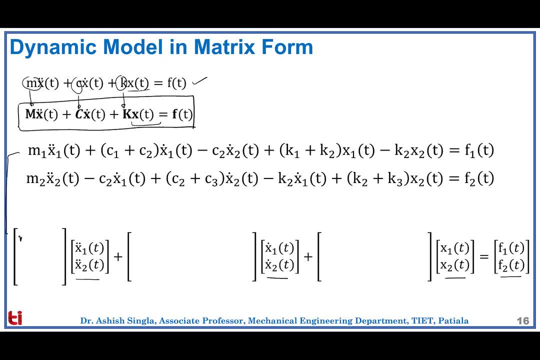 So here you can see, from the first equation we can see M1, X1 double dot. you have the contributions from the X1 double dot, So we can write M1, and there is no contribution from the X2 double dot term, so that is 0.. 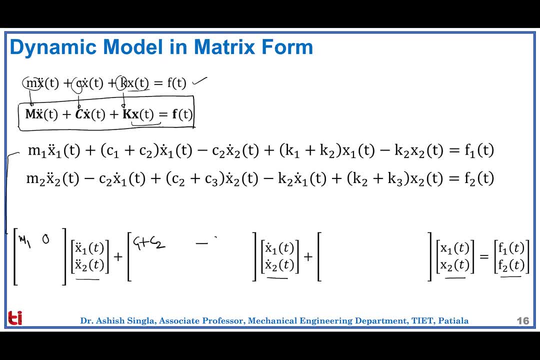 So then we have: for velocity, we have C1 plus C2.. This is a contribution from X1 dot. So then we have minus C2 contribution from X2 dot. this is a contribution from x1 side, and then minus k2, this is a contribution from x2 side. 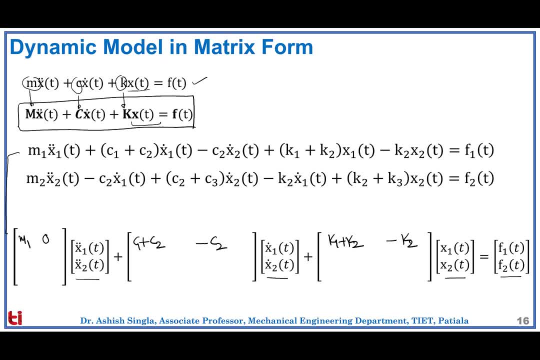 is equal to f1 of t. So that is the first row of the matrices which comes from the first equation of motion. So then comes the second row of this matrix which belongs to the second equation of motion. Here you can see there is no contribution from x1 double dot, so that term goes to 0. 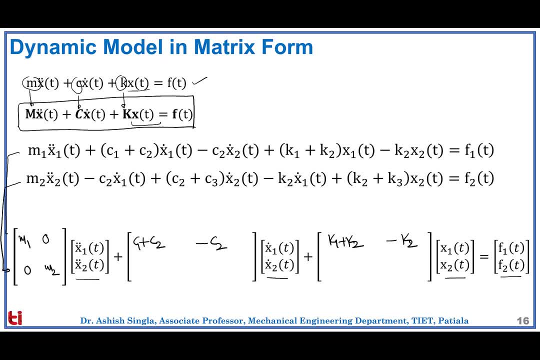 and the second term is m2.. So then we have x1 dot here we have minus c2, and then x2 dot term, we have c2 plus c3.. So then we have x1, which is equal to minus k2 over here, and then we have x2. 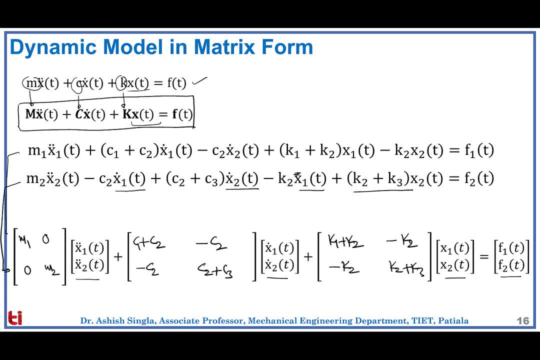 which is equal to k2 plus k3. and finally, this f2 is already written over here. So this is the way we can write the matrices. So this is the way we can write the matrices. So this is the way we can. 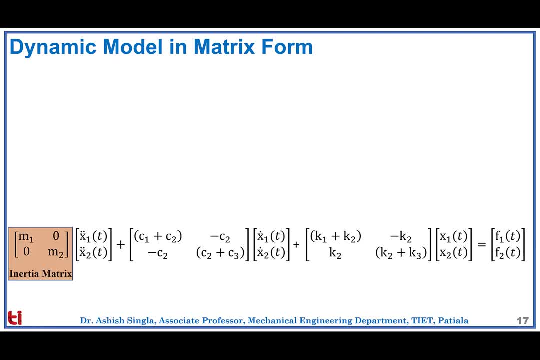 the final matrix, which is called as the inertia matrix. The next matrix, containing all the coefficient of damping elements, is known as the damping matrix, and the third matrix, containing all the stiffness, is called as the stiffness matrix. So this vector is containing all the displacement- is called as vector of displacements and the vector containing all the forces. 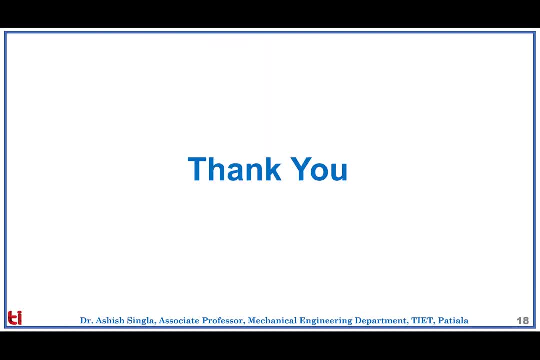 is called as the vector of forces. Thank you.